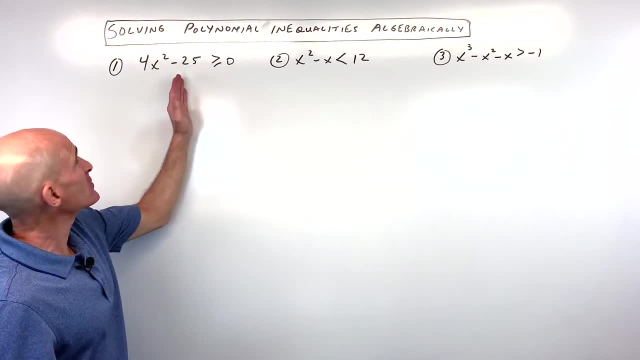 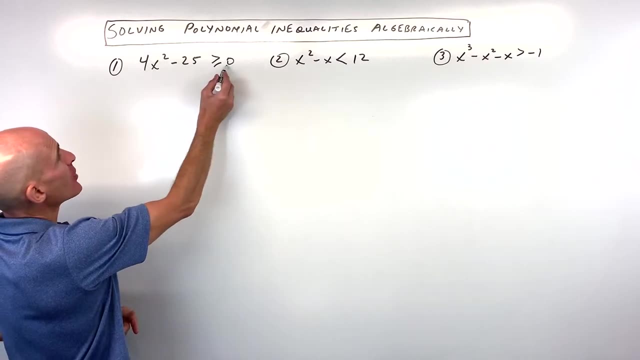 three examples: See if you can do some of these on your own. but the first thing we want to do, like I said, is get everything on one side, set it to zero, and then we want to factor it as much as we can. So what I notice here it's already zero on one side. but this is what we call a difference of. 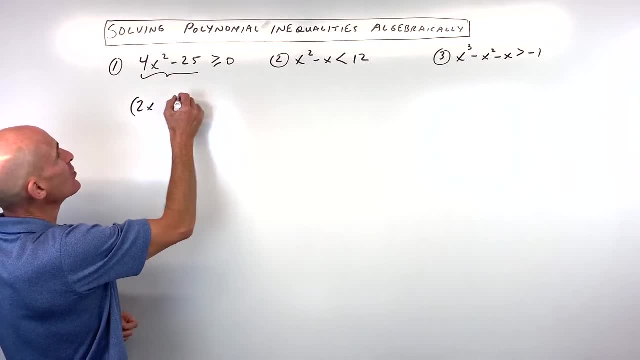 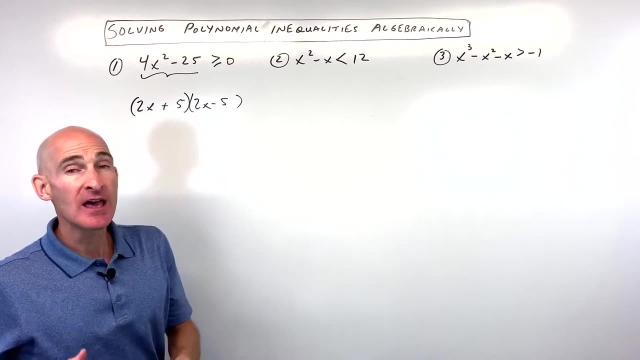 two squares. So 4x squared is a perfect square because 2x times 2x 25 is a perfect square because 5 times itself. One of these is positive, one of these is negative. If you need to review factoring, check out my factoring video where I talk about how to factor all different types and 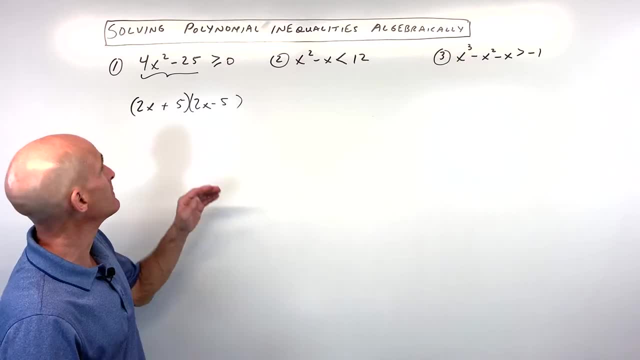 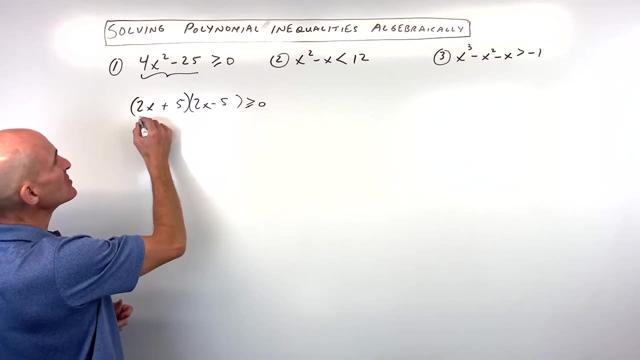 how to recognize them, and I show a nice tree diagram so that you can make the decision about what to do: first, second, third. But now what we want to do is we want to set each of these factors, each of these groups, to zero, So you can make a little mini equation, or 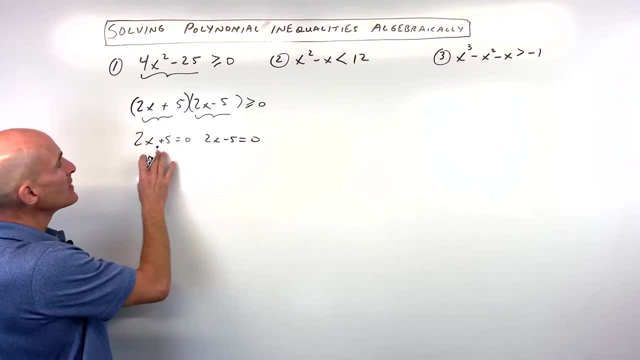 you can do the work in your head if you're good at that. So here I'm going to subtract 5 from both sides and I'm going to divide both sides by 2.. So we get x equals negative five halves. Here I'm. 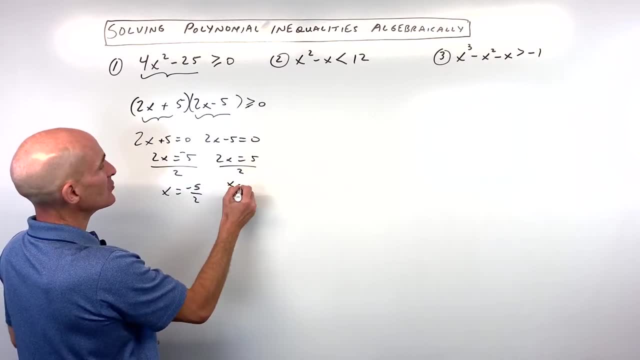 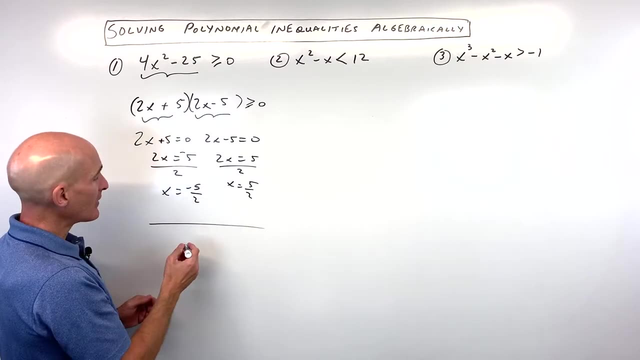 going to add five to both sides and divide both sides by two. so we get x equals positive five halves. Then what you want to do is you want to go to the number line and you want to plot these on the number line from lowest to highest, So the smallest to the highest, So the smallest to the 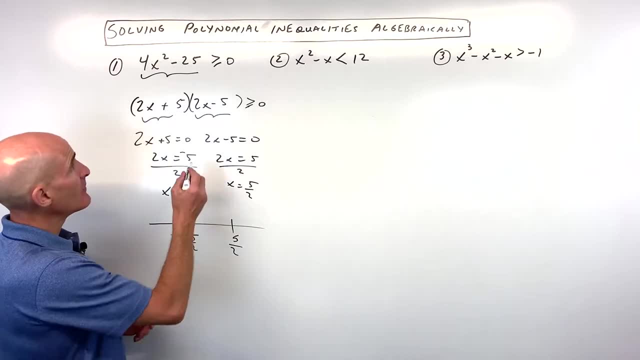 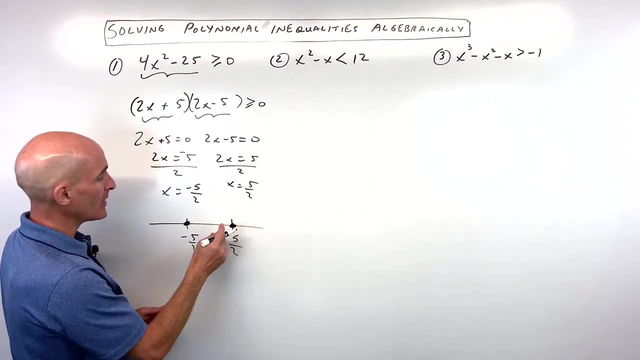 on the left and larger one on the right, and because it's greater than or equal to zero. equal to means this is going to be a closed circle. it's going to be, it's going to include that point. so right at negative five halves or positive five. 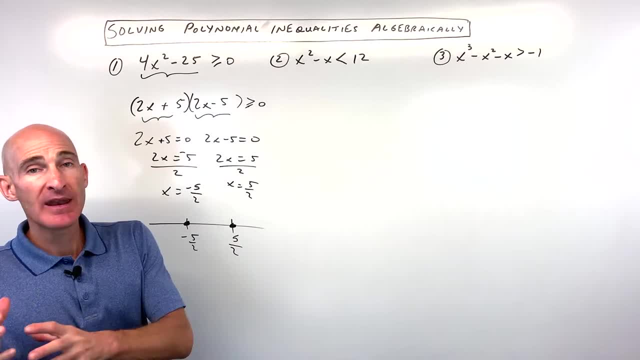 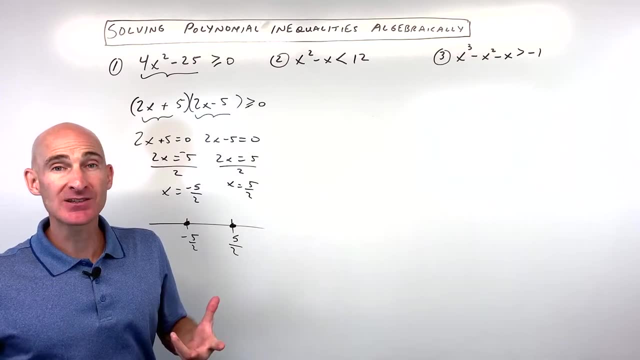 halves. that's going to make the left side equal to zero. but now we want to see what points are going to make it greater than zero. greater than zero is another way of saying making it positive, right? so we're going to do something called sine analysis, and what you do is you just pick a point in each of these. 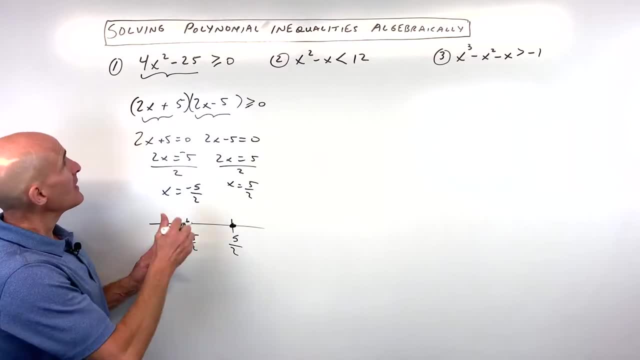 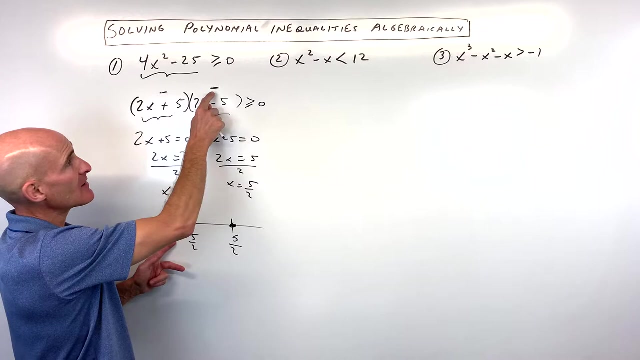 intervals. so, for example, maybe negative three over here. if I put negative three in for X, I get negative. six plus five is negative one, but I'm just going to call that negative, okay. negative three times two is negative. six minus five is a negative eleven, that's also negative. a negative times a negative is a positive. 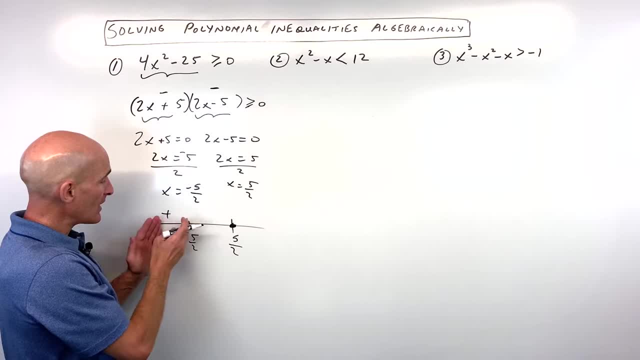 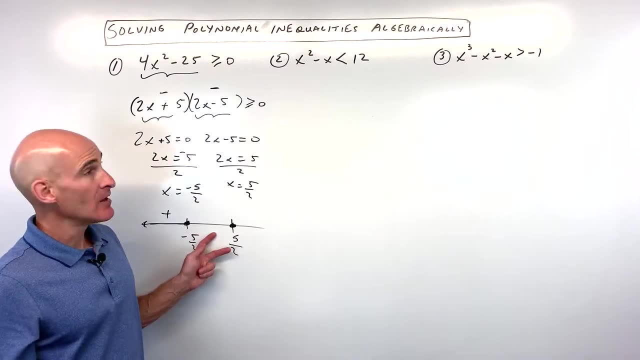 so I'm just going to put a plus sign there. so any point in this interval, okay, all the way to negative infinity, it's going to be positive. let's pick a point in this interval. how about zero? if I put zero in? two times zero, zero plus five is five. that's positive. two times zero is. 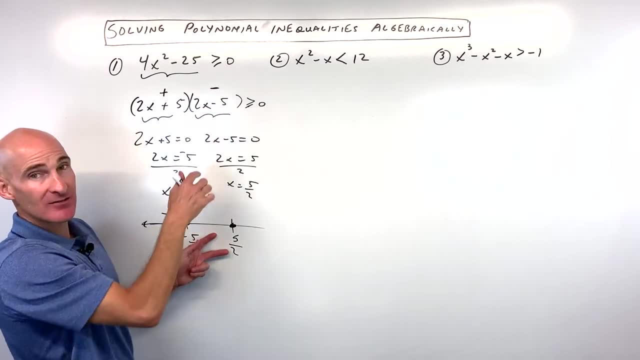 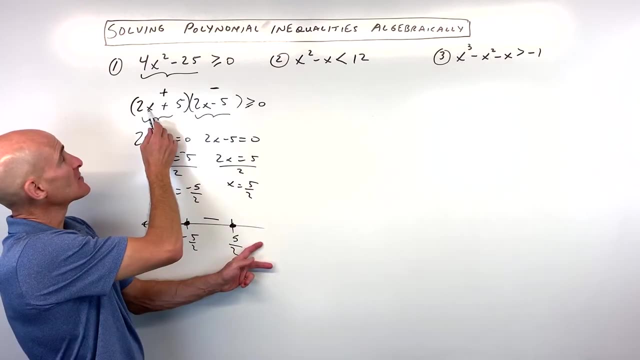 zero minus five, that's negative. a positive times a negative is a negative. so I'll put a minus sign or a negative there. if we pick a point over here. say like positive three two times three is six plus five is eleven. that's positive. two times three is six minus five is one. that's also positive. a positive times a. 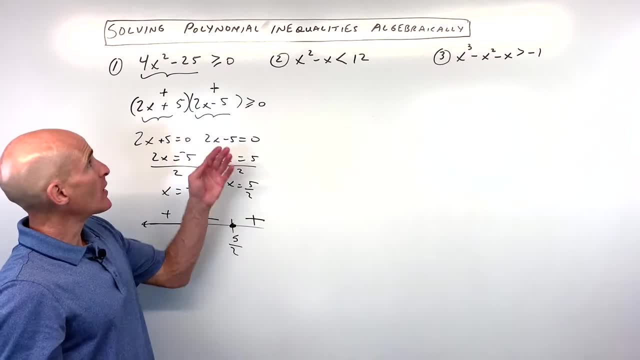 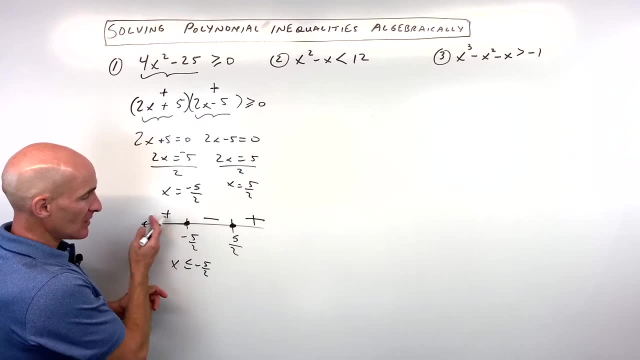 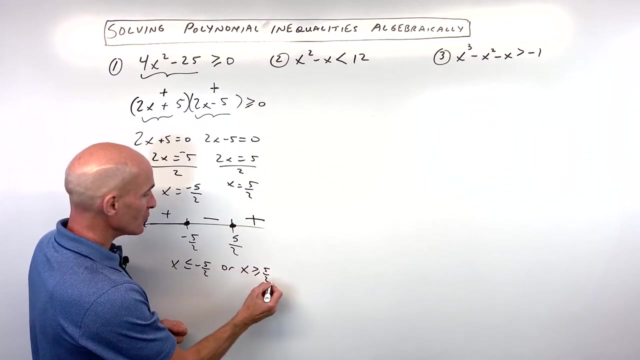 positive is a positive. so now we can see. we want to know where it's greater than or equal to zero. so it's going to be when X is less than or equal to negative five halves. okay, or now, in math, remember, or means union, it means both: X is greater than or equal to five halves. so you're. 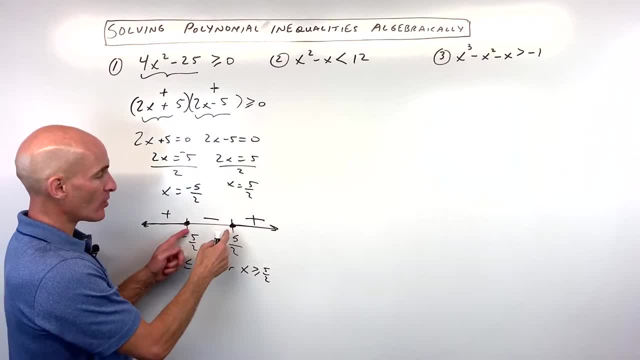 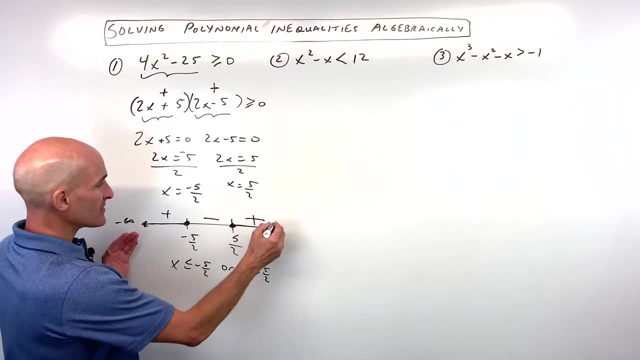 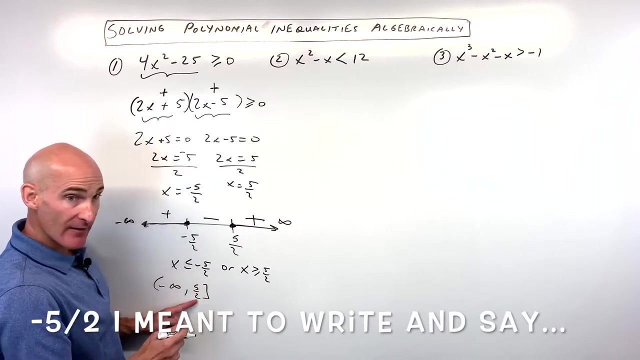 going to be to the right of this point or to the left of this point, or it'll equal zero right at those points. now, if you know interval notation, we're starting over here at negative infinity. this is positive infinity, so it's going to be from negative infinity all the way to five halves, including five halves, so I 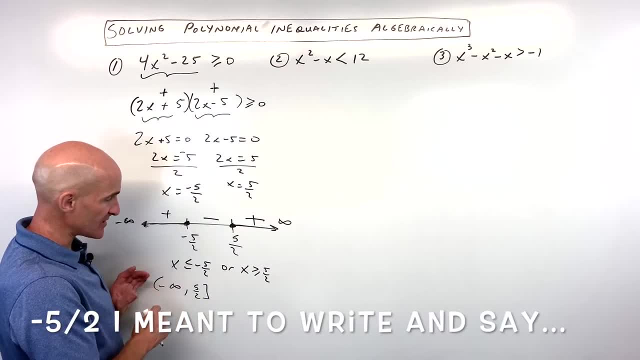 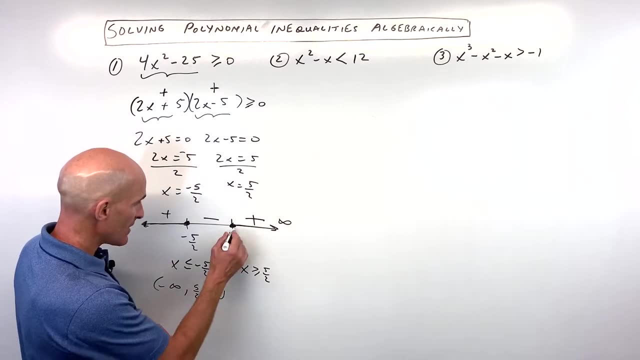 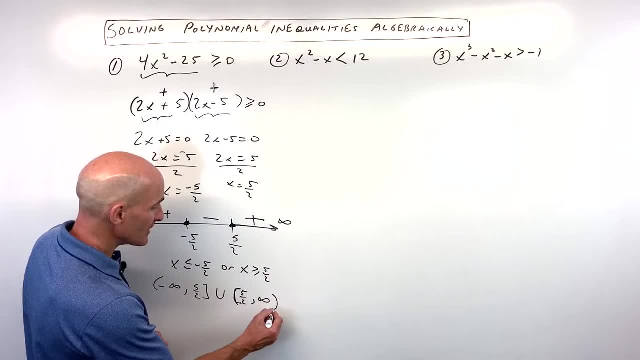 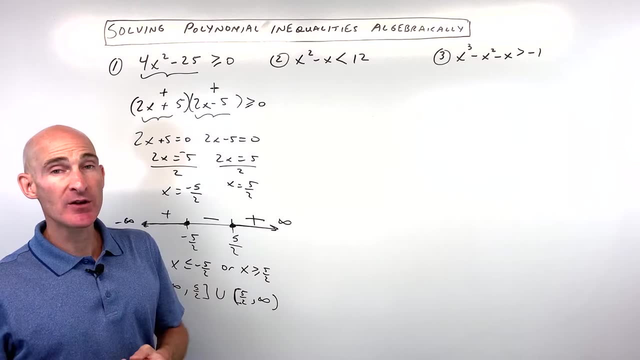 bracket because it includes five halves all the way to positive infinity, can never reach infinity. that's open, okay, with the parentheses. so interval notation or inequality notation, whichever way your teacher prefers. now you might be saying: Mario, you know, I don't really understand what all this is. 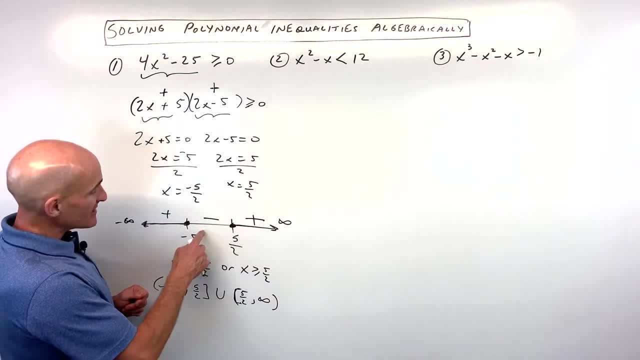 about right. and here's the. and I understand. see, the thing is, if we were to graph this, and not one dimension, but in two dimensions, like on an XY coordinate plane, okay, like, see, this is zero here, this is your origin- you would have a parabola that would 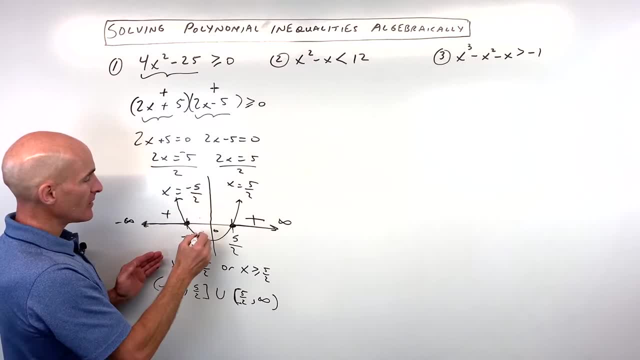 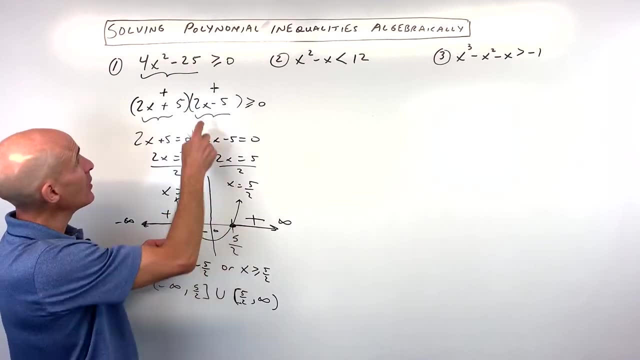 look something like this, okay, roughly, and so what you can see is it's basically saying: like: where is the parabola? equal to zero, that's right here- at these X intercepts, or greater than zero, meaning above the x-axis, and that's going to be. 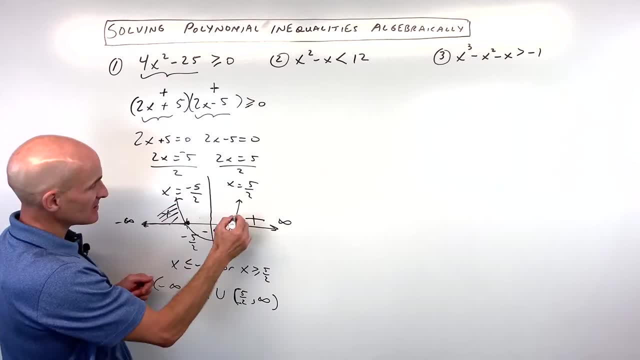 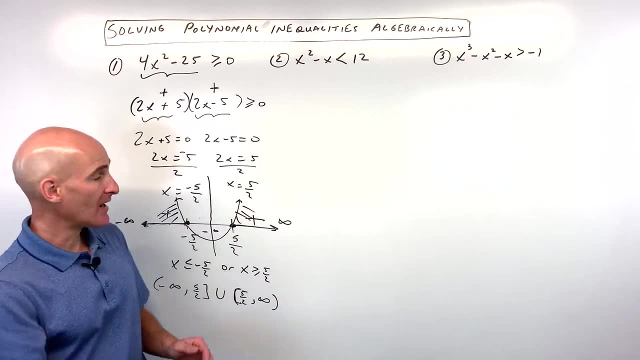 when you're to the left here, see how you're above the x-axis over here. you're below the x-axis right, but what we're doing is just a quicker way, just analyzing it in one dimension- okay, on the number line- as opposed to going through all the trouble of graphing the whole graph and seeing. 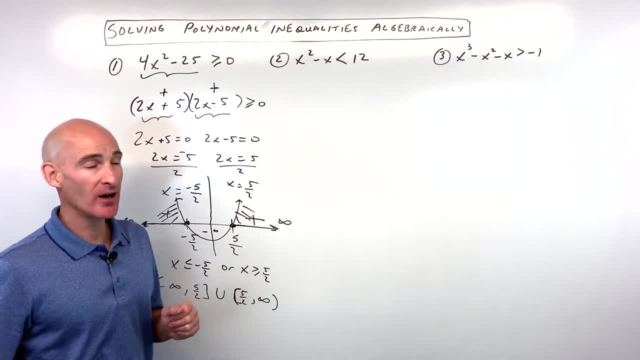 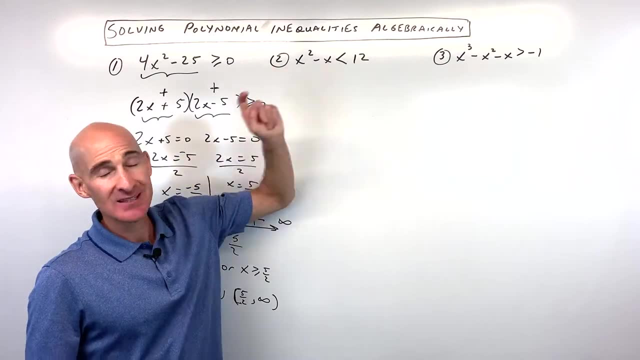 where it's above the x-axis or equal to you know, right on the x-axis. let's look at another example, see if you can do this one. so for number two, we have x squared minus X is less than 12, okay. so remember step number one, get everything. 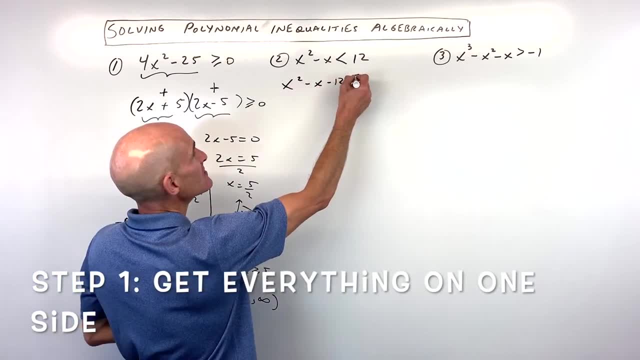 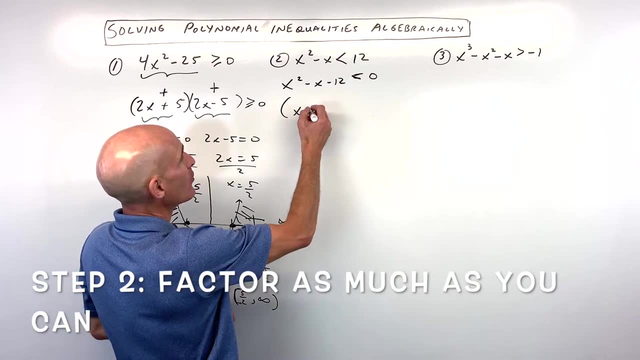 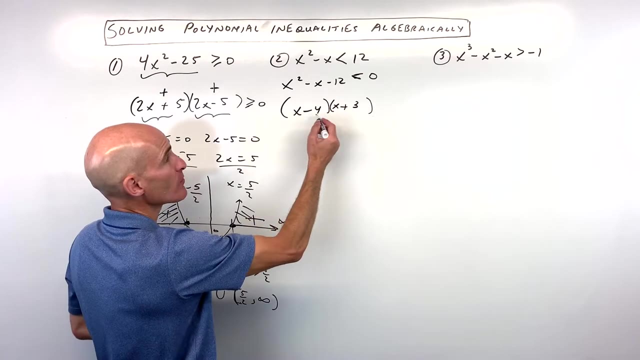 on one side and set it to zero, right. okay, step number two: factor as much as you can. so what multiplies to negative 12 but adds to negative 1, that's negative 4 and positive 3. you can check your work by foiling this out and make sure it comes out to the original. 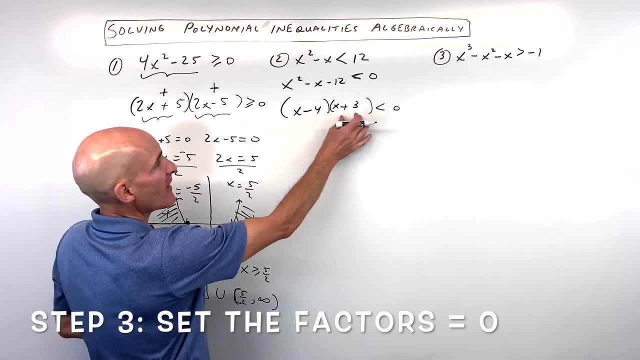 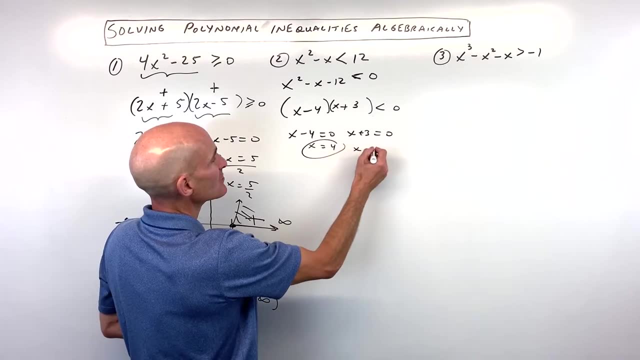 there. step number three. we set each factor to zero. so we make a little mini equation: add 4 to both sides, subtract 3. X equals negative 3, and then step number. what are we on step number 4? we plot it on the number line from: 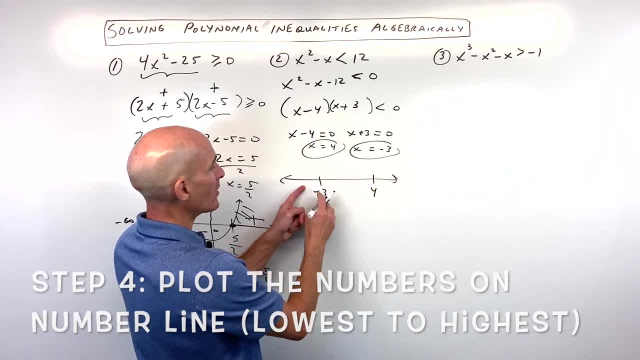 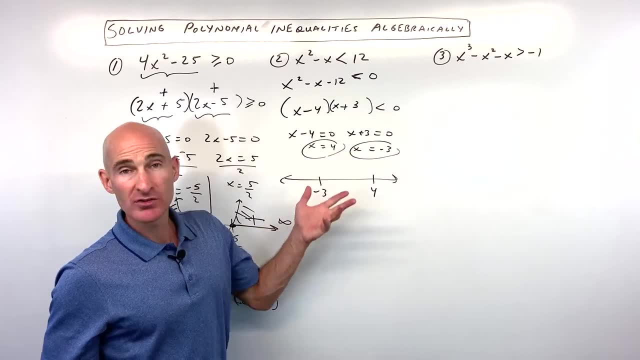 lowest to highest, so from negative 3, 4. you don't want to reverse and I make sure if the lowest number all the way to the highest number and you could, when you factor, you could have more than two solutions here. you can have 3, 4, 5. 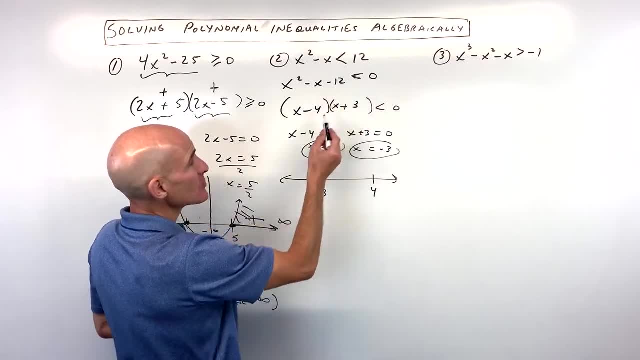 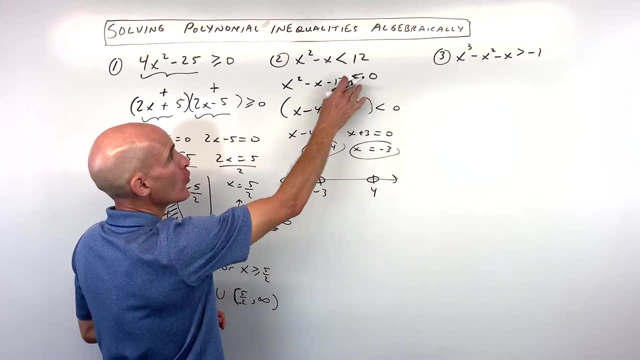 however many, but now in this one, see how it's less than 0 but not equal to 0. so that means that these are actually going to be open. okay, because we want to know where it's going to be less than 0, meaning below the x-axis, not on the x-axis. 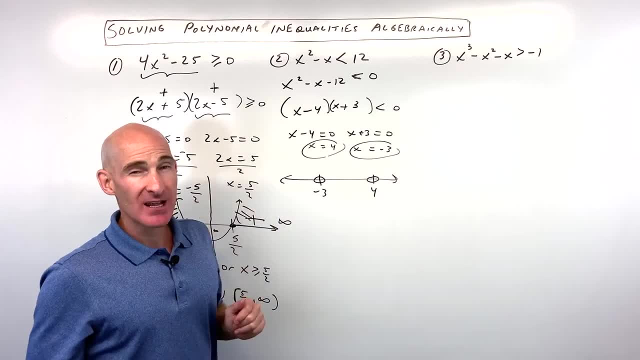 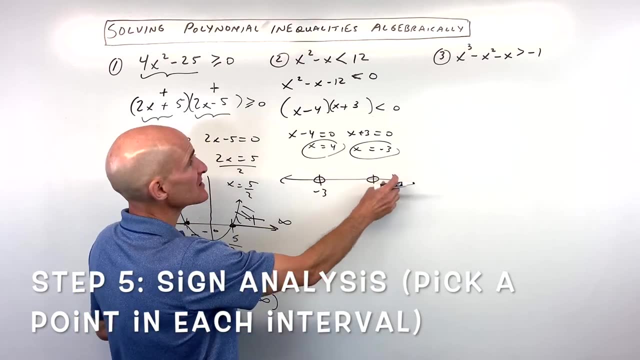 if we were to graph it like this in two dimensions. so now we're on step number 5, I believe we're gonna do the sine analysis, okay, and we're gonna pick some test points in each interval to see if it where it is negative, because we wanna know where it's less than 0 pick. 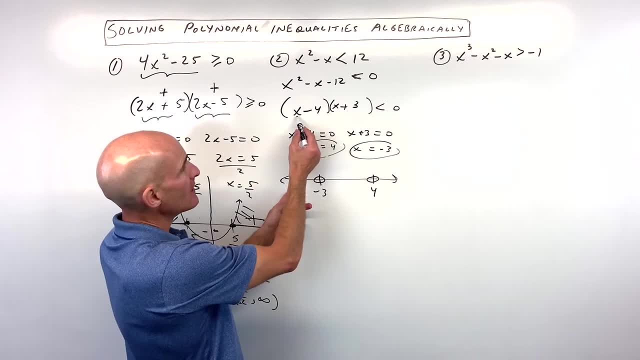 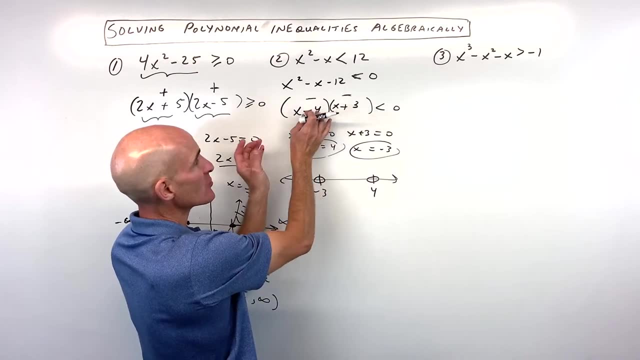 easy numbers. a good number here might be like negative 4. negative 4 minus 4 is negative 8. I'll just say negative. negative 4 plus 3 is negative 1, that's negative. see how these two parentheses are right next to each other. they're. 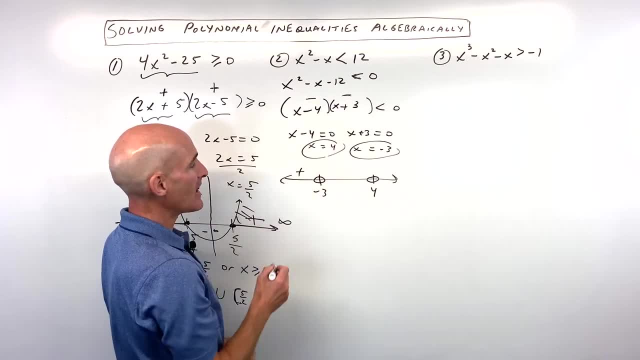 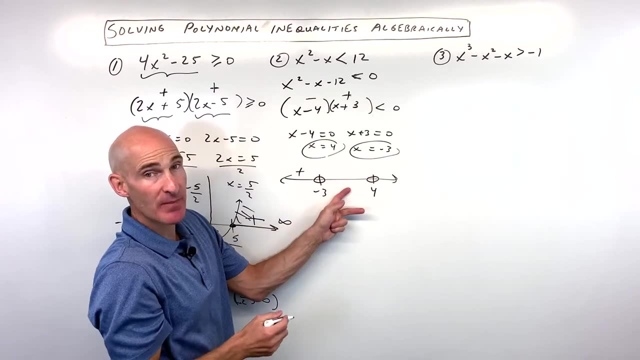 multiplied together. and negative times a negative is a positive if we pick, let's say, 0. 0 minus 4 is negative, 4 that's negative, 0 plus 3 is positive, 3 that's positive. a negative times a positive is a negative if we pick a number over here. 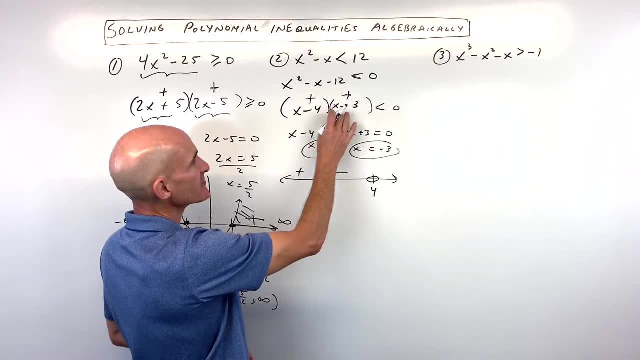 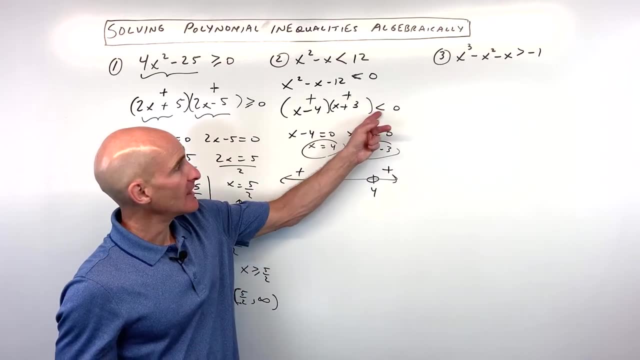 say like 10, 10 minus 4 is 6, that's positive, 10 plus 3 is 13, that's positive and a positive times a positive is a positive. but we're looking for where the graph is less than 0, meaning you know, below the x-axis, or where it's negative. 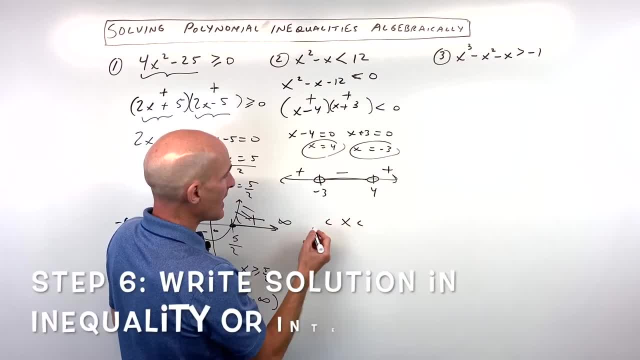 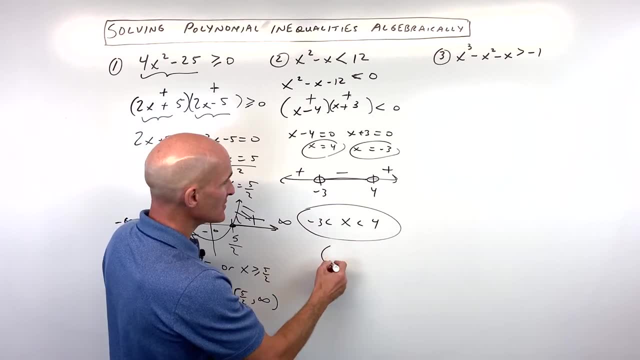 so that's going to be right here and you can write this as a compound inequality X is greater than negative 3 and less than 4. ok, that's one option. or if you want to use the interval notation from negative 3 to 4, you can check out my video about the difference between inequality. 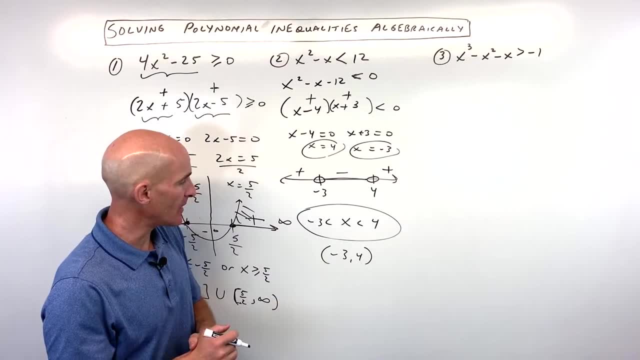 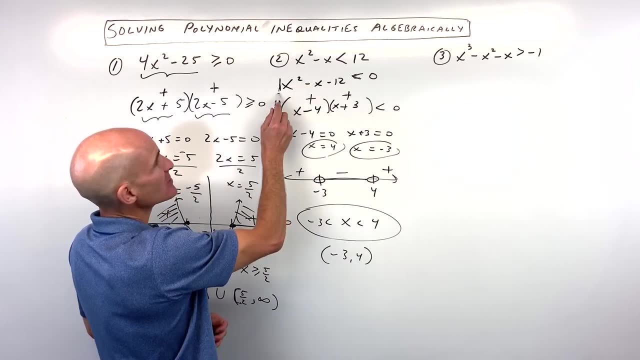 notation and interval notation. if this is challenging for you, just look that up on YouTube now if you want to understand the set on deeper level. remember, this is a parabola. see how this value is positive one that means this graph is going to be opening up. it was like a negative and the opening down. so we know. 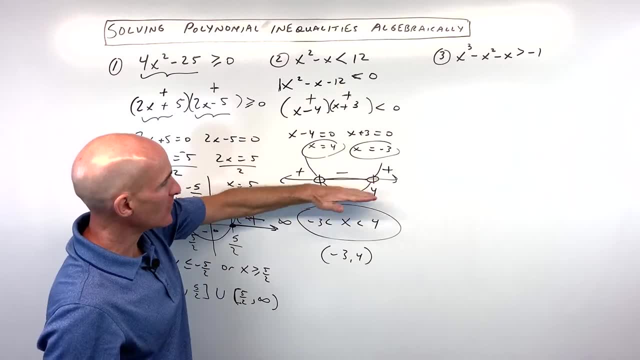 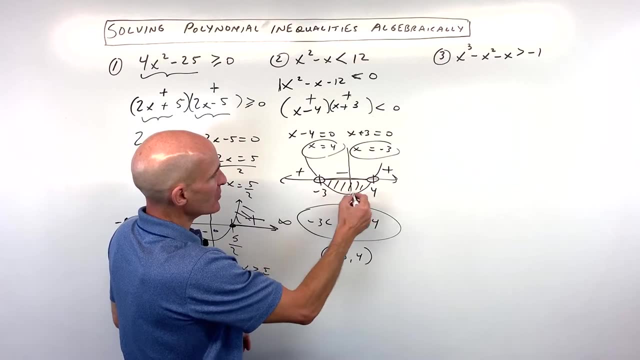 the graph looks like that. we're saying: where is it less than 0, meaning where's it below the x-axis and the y-axis would be somewhere here, but you were looking for where it's below, not equal to, because it was less than but not equal. 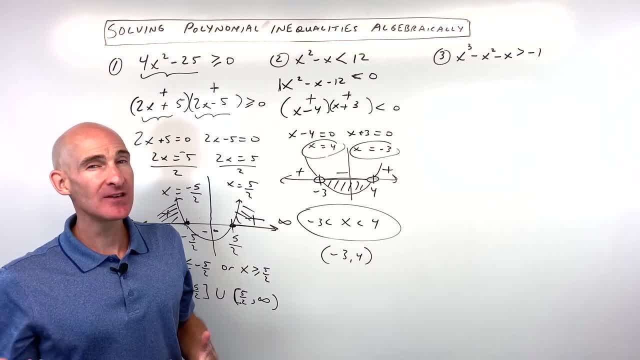 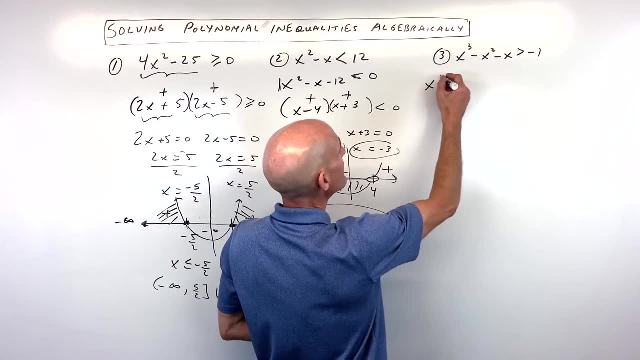 to zero and you got it. so a third example: see if you can do this one on your own. this is a little bit more challenging. I try to start easy and get progressively more challenging. you've probably noticed that if you've been watching my videos, and I also wanted to say if you like my teaching style, you 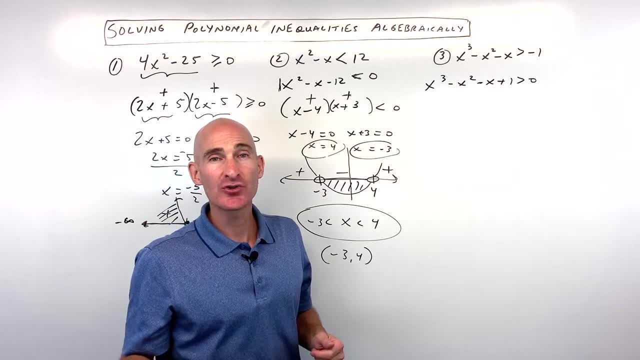 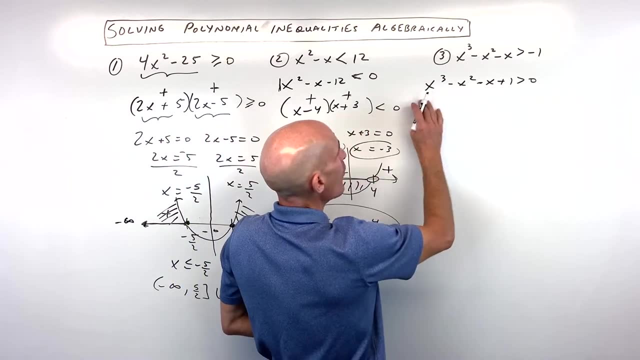 know I've got courses. I've got algebra 1, algebra 2, geometry, ACT math, SAT math. so those are for sale. check those out. I'll have a link in the description. but what do you notice about this one? here we've got four terms right, so we could try. 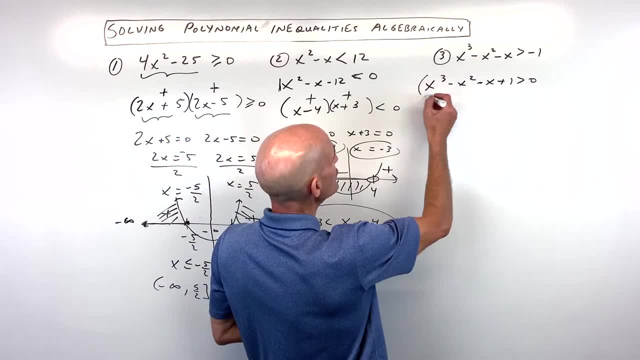 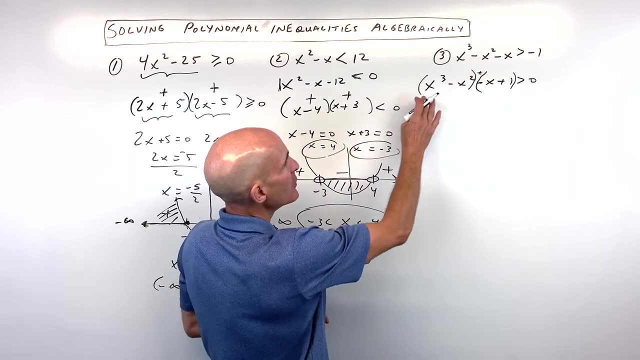 factoring by grouping. you know you're factoring by grouping. you group the first two terms, put a plus sign there and you group the last two terms. okay, then you factor out the greatest common factor, so in this case it's x squared. and then you factor out the greatest common factor, so in this case it's x squared. 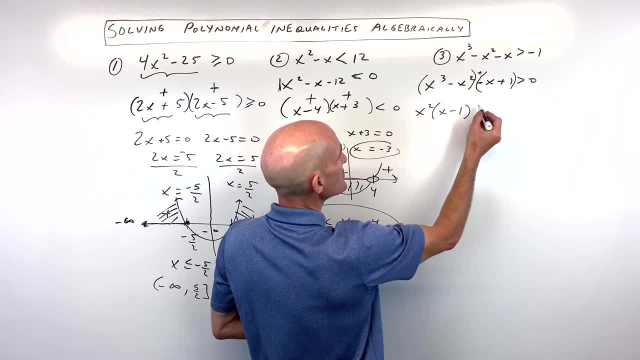 and then you factor out the greatest common factor. so in this case it's x squared. okay, so I divided these both by x squared this one because it starts with a negative. I'm going to factor out a negative 1 out of both of these guys. see. 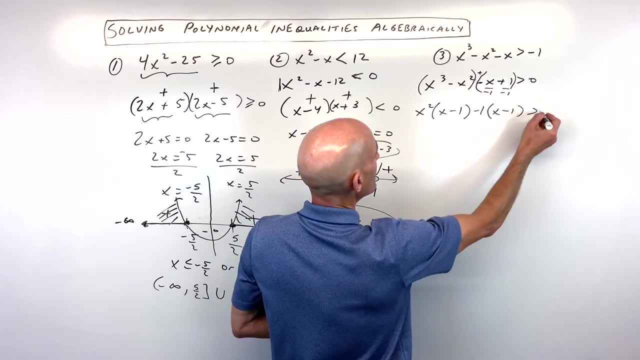 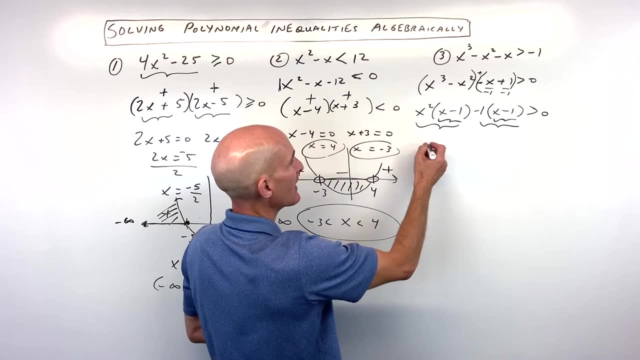 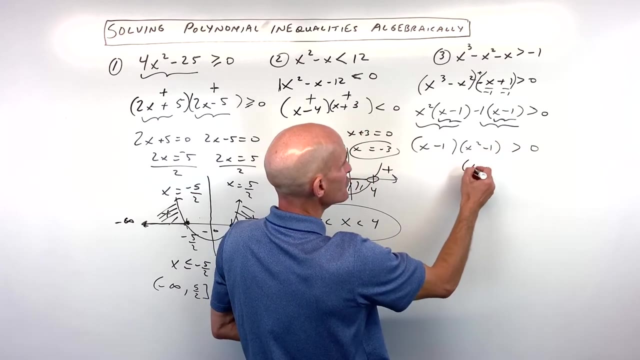 like that. so positive 1 divided by negative 1 is negative 1. and now, because we have an x minus 1 in common in both of this group here and this group here, we can factor out that x minus 1 and we're left with x squared minus 1. but this is a difference of two. 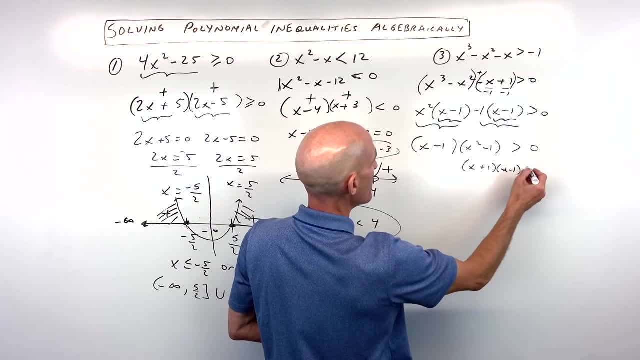 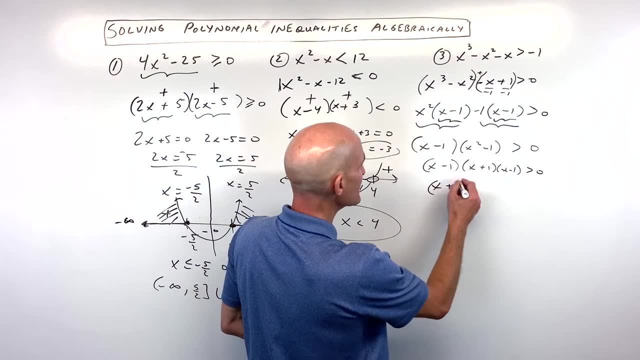 squares, so we can factor that further x plus 1, x minus 1 and bring down the x minus 1. now you notice that there's an x minus 1 and an x minus 1. we can condense this and write this as x minus 1, the quantity squared. 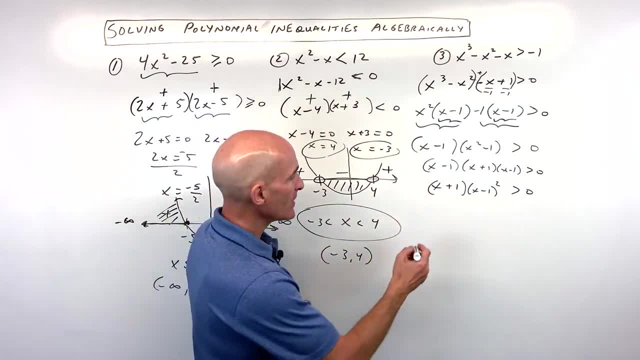 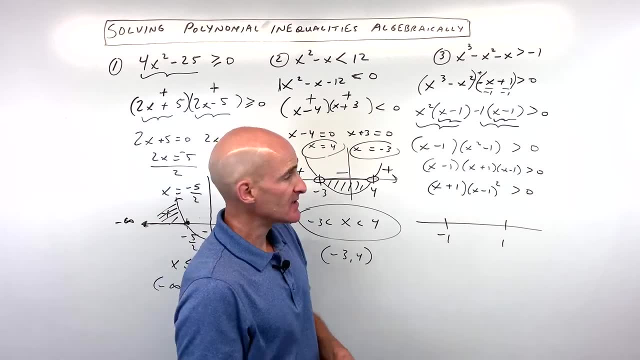 okay, but now when we set these groups equal to 0, we get negative 1 and positive 1. we want it to be greater than 0, so that means that these are going to be open. okay, if it was greater than or equal to 0, then these would be closed. 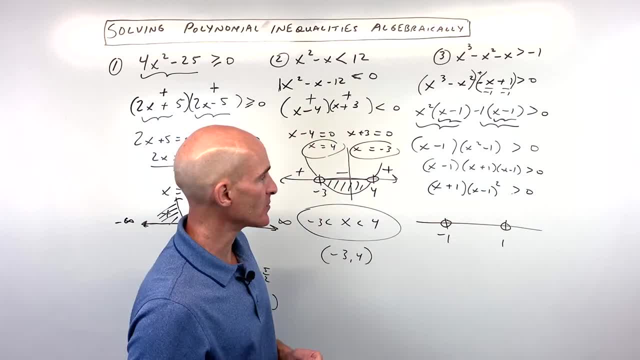 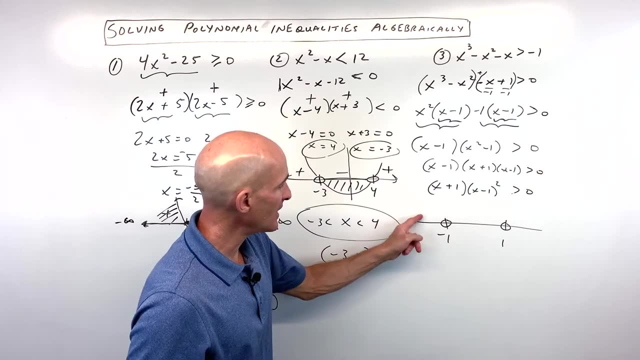 because at these points that's where it crosses the x axis, that's where it's equal to 0. now we just have to do our test points and I'm going to pick negative 2, 0 and positive 2. so if I do negative 2, I get. 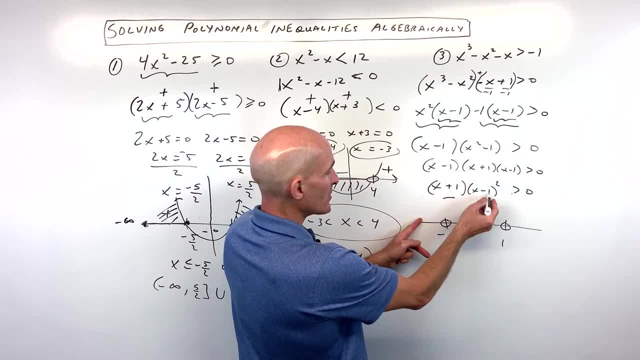 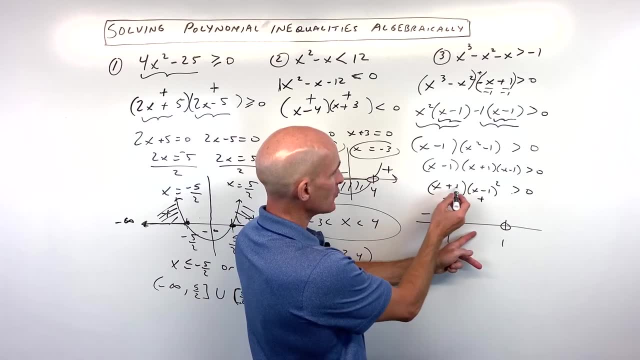 negative, 2 plus 1 is negative 1, and negative 2 minus 1 is negative 3, but negative 3 squared is positive 9, right? so negative times: a positive is a negative. if I do 0, 0 plus 1 is positive 1, that's positive. and one thing to: 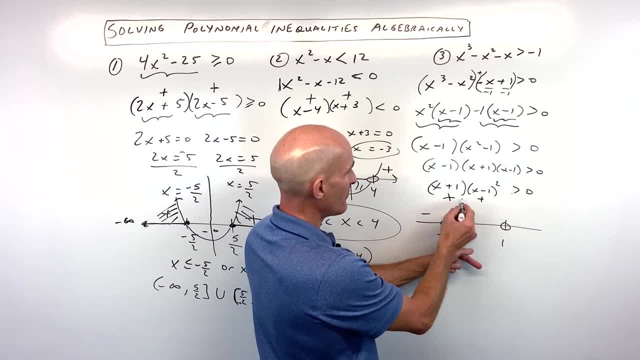 notice here is: whenever you square something, it's always going to be positive. so we have a positive times, a positive which is a positive, and if we do 2, we get 3, which is positive. 2 minus 1 is 1. 1 squared is positive, and 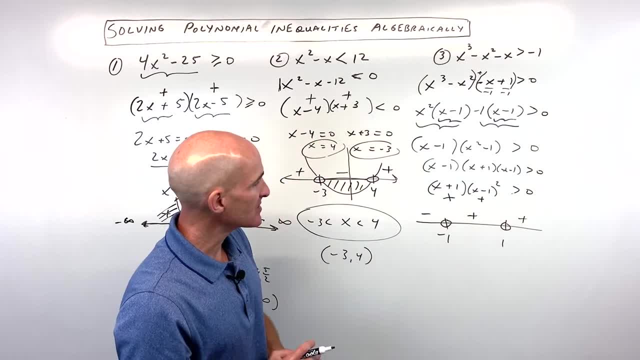 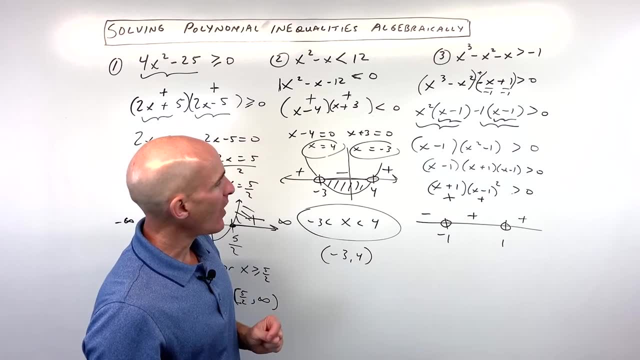 a positive times. a positive is a positive. now you're probably saying, Mario, this is a little bit unusual, right, because you've got a positive and a positive over here. they seem to always alternate. and you're probably wondering: well, why is that? well, if we were to graph this in two dimensions, like an XY. 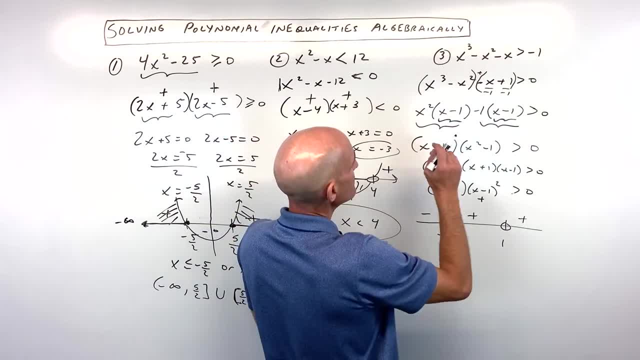 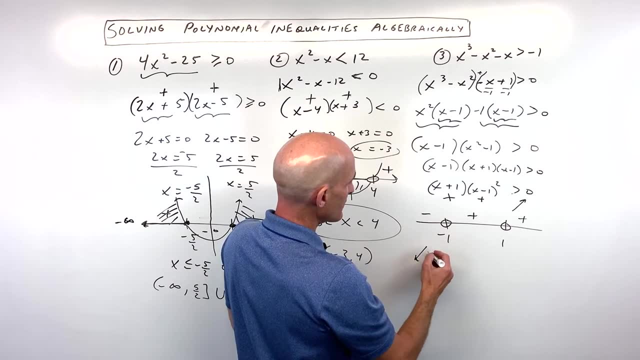 coordinate plane notice. this leading coefficient is positive. that means it's going to be going up to the right, like this, and it's an odd degree, which means it's going to be going down to the left, like this. so this graph is actually going to look something like this. 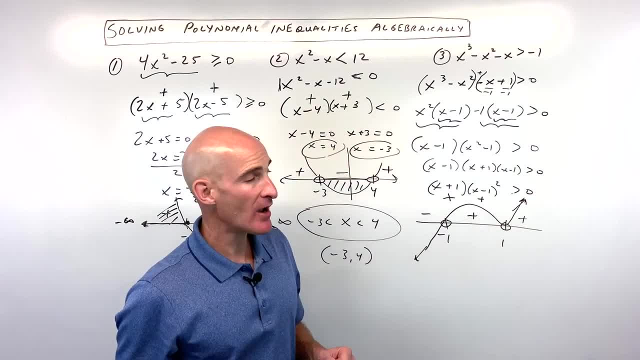 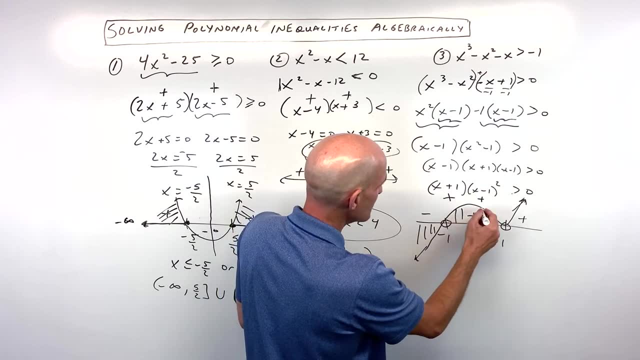 and it's going to bounce right off one, and you can check that by graphing this on your graphing calculator. but notice how it's below the x-axis here. see how we got negative. it's above the x-axis here. you got positive and it's also. 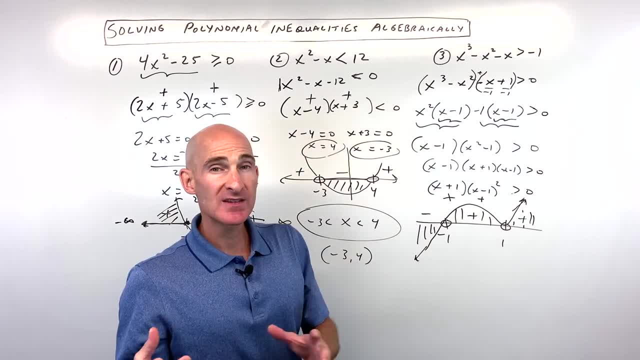 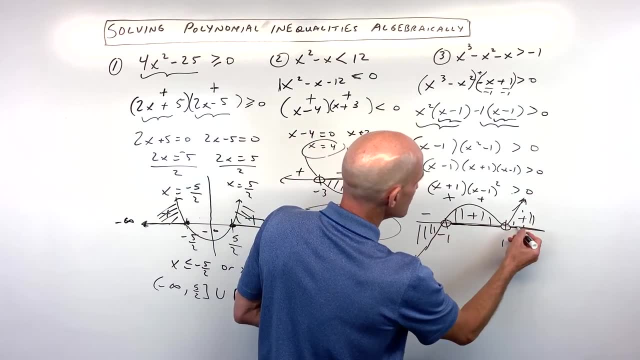 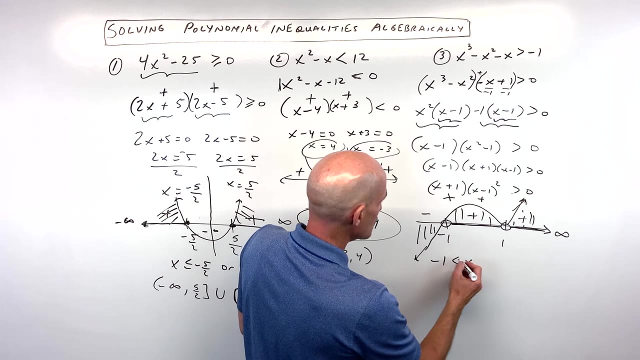 above the x-axis here, positive. so if we want to write this in inequality notation, we want it to be greater than zero, so where it's positive. so we want this interval right here as well as this interval right here, okay, going to infinity, but we don't want this point one. so I'm going to say X is greater. 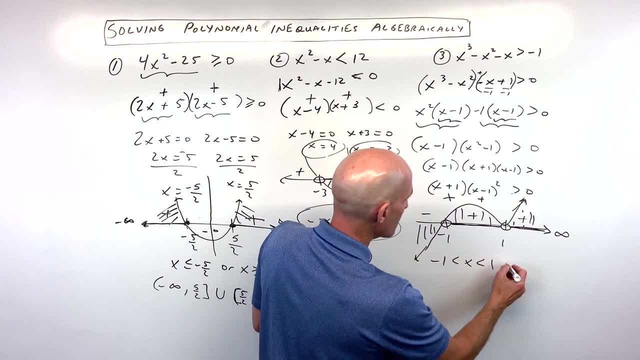 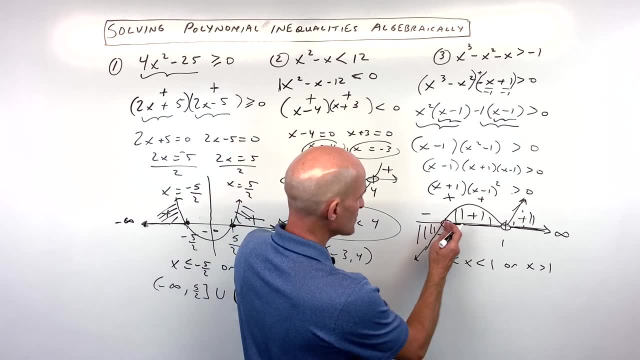 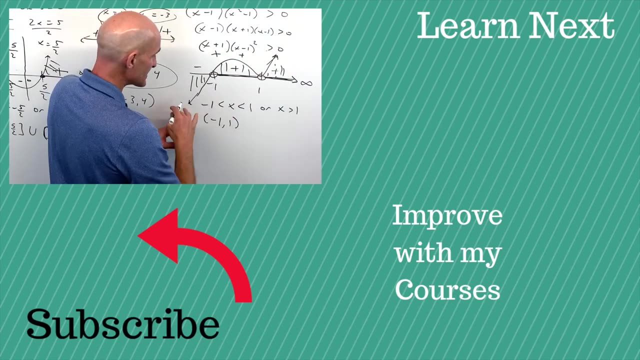 than negative one and less than one. okay, or remember. or means Union. it means both. in math, X is greater than one. if we want to do the interval notation, we start on the left. we work our way from left to right. negative one to one. notice these are parentheses or open means. it does include the. it does not include the. 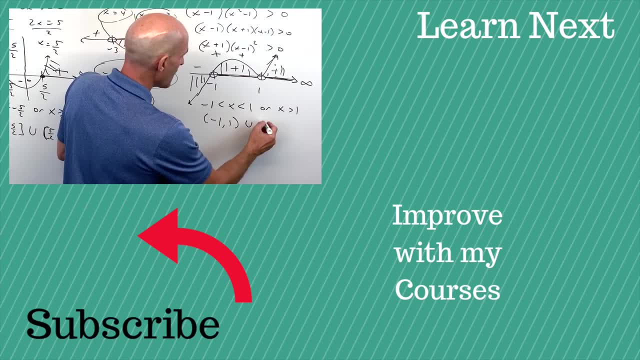 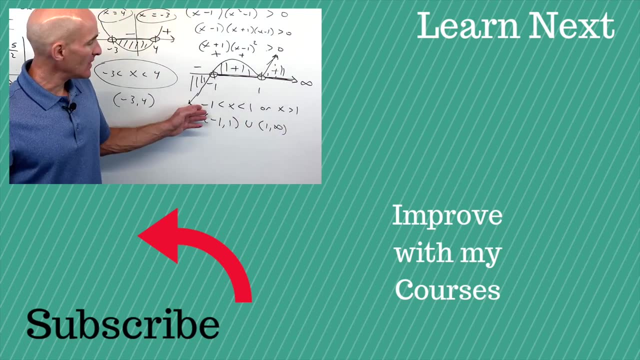 endpoints Union. okay, U for Union one. two positive infinity. so again open, because it doesn't include one infinity. we can't really reach infinity, so inequality or interval notation, either one. great job, I'll see you in the next video. 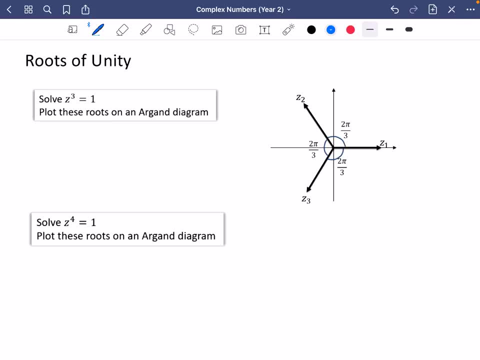 Okay, we're going to continue with exercise 1f, And the second part of this is to do with something called roots of unity. Now, roots of unity- unity makes you think of one, So roots of unity are equations that are in the form z to the power of n equals one. So what? 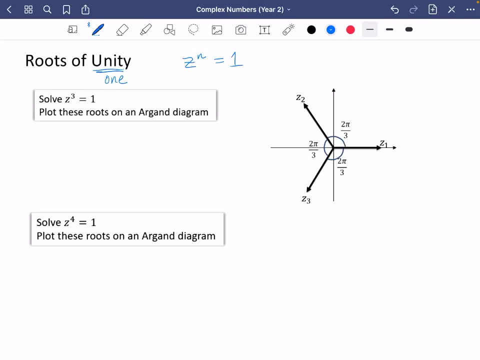 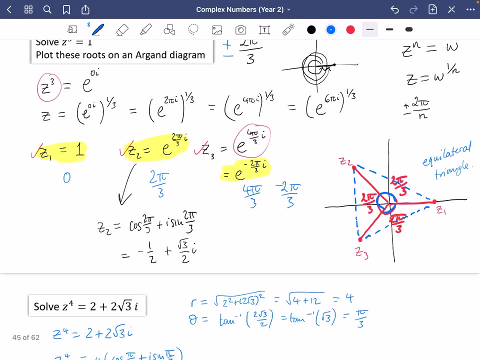 are the roots of one. Now it's really interesting. we've actually already worked out some of the. we worked out the cube roots of one earlier on And obviously one of them was just one. I think the second one that we had from earlier was a half plus root 3 over 2i, so that's. 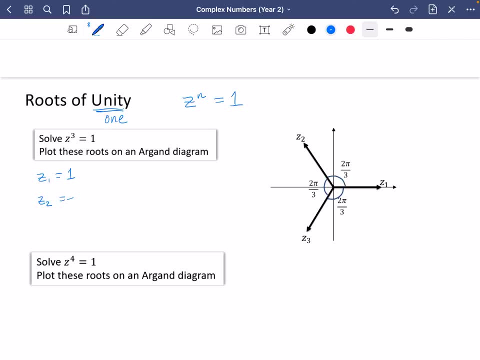 minus half plus root 3 over 2i, And you can see which one this is corresponding to, because it is minus a half plus root 3 over 2i. And you can also do the same thing with the other ones, like which one is the half plus.